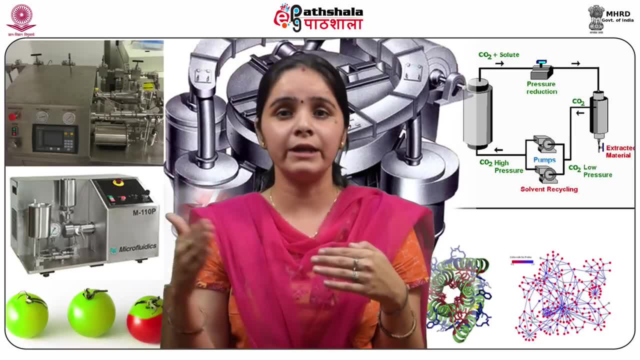 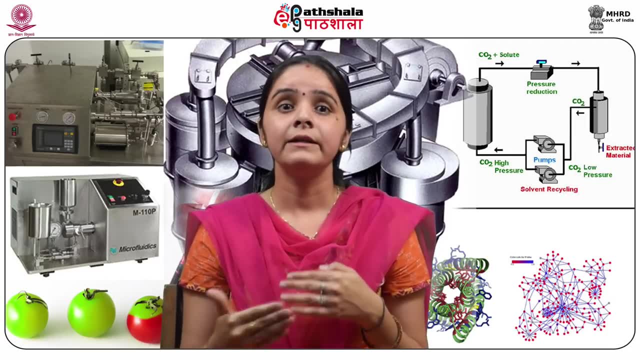 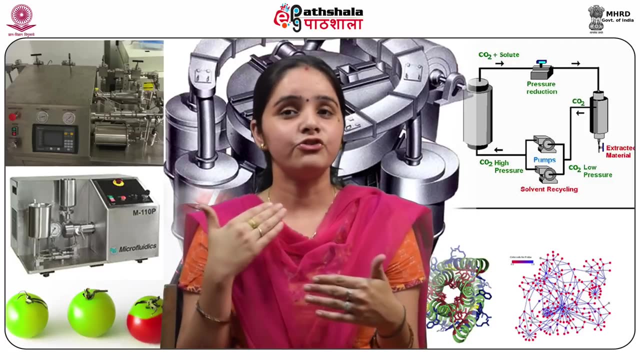 of the solute through the liquid boundary layer. Therefore the solute is released and любits the solution of the solution. Ideally extruded solution is rapidly extracted. It should be simple and inexpensive in nature. It should give a quantitative recovery of analyte without loss or degradation. It should 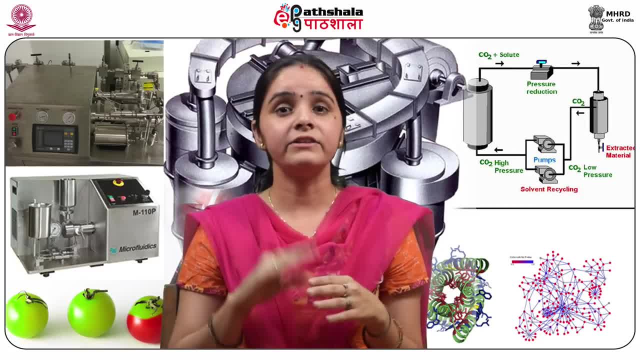 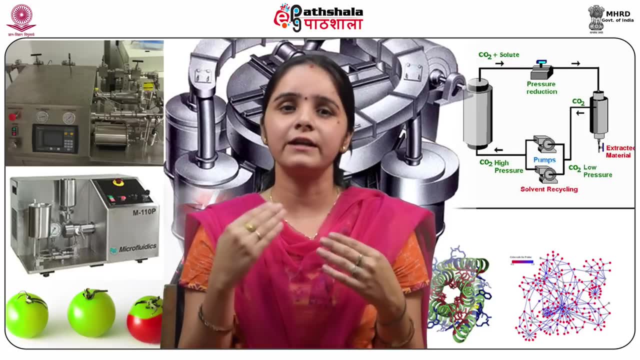 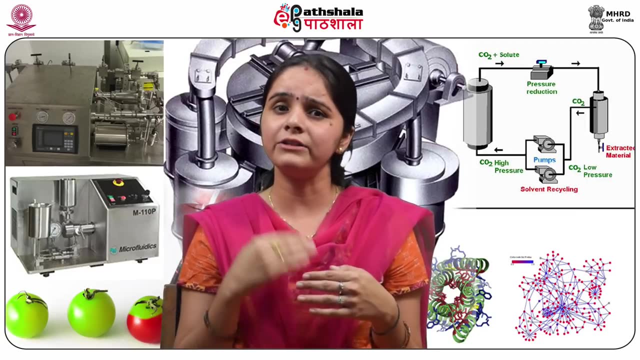 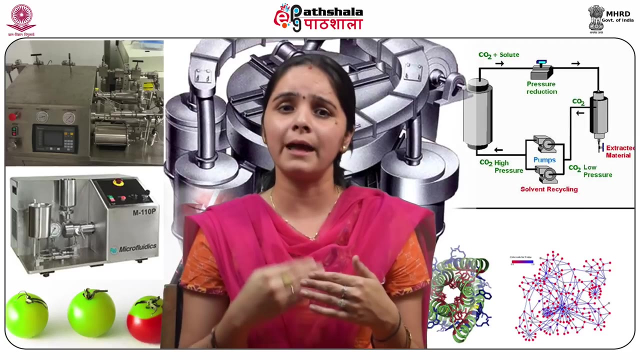 yield a solution of the analyte that is sufficiently concentrated to permit the final measurement without any further concentration. also, one important requirement is that it should generate a very little or no laboratory wastage that have to be disposed of. the most common method of extraction of the sample is using a 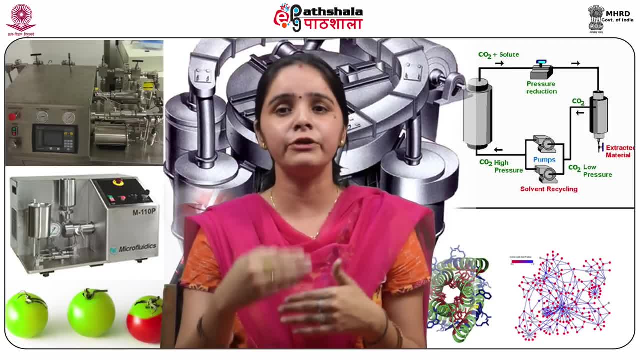 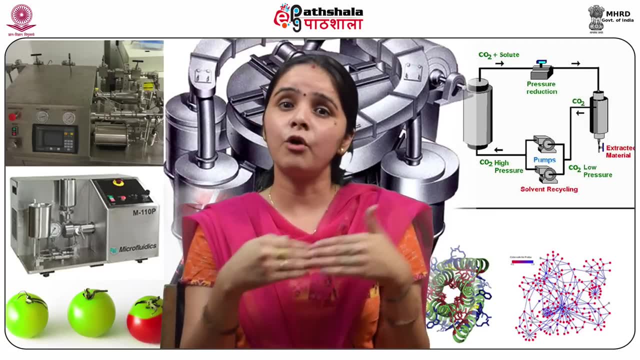 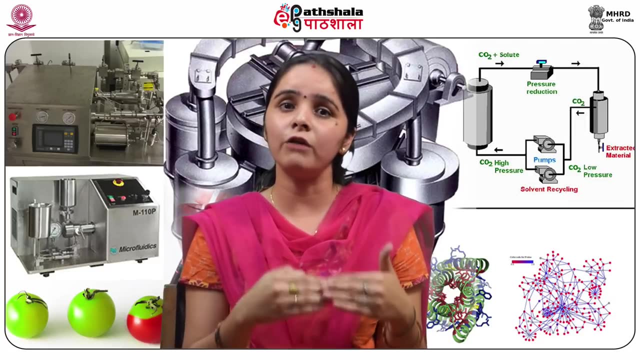 sock slate extractor with the help of different organic solvents. these organic solvents are hydrocarbons and chlorinated in nature. then what is supercritical food extraction? it is similar to the sock slate extraction process, but here the solvent is supercritical fruit. the advantage of this? 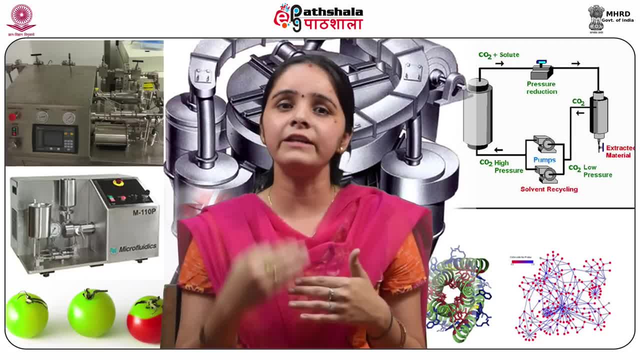 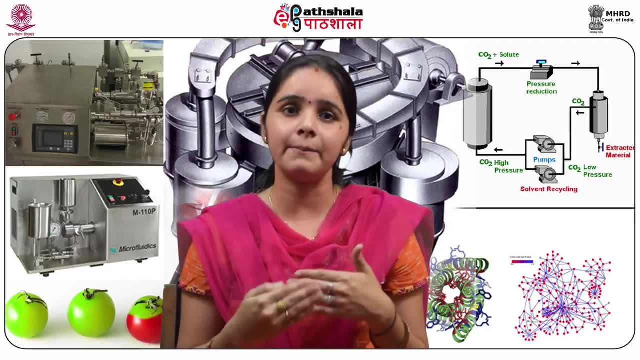 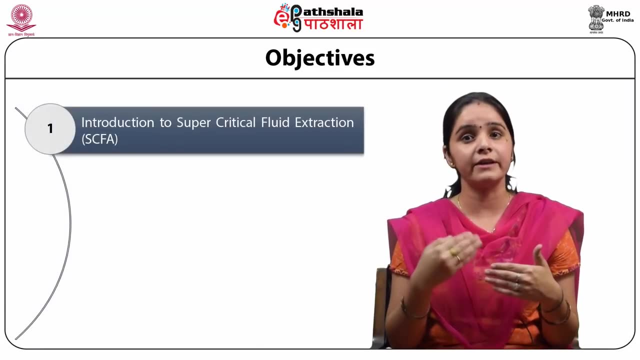 supercritical food extraction is that it is a green technology, means it results in the waste material that can be easily recyclable and usable. so in this module, So in this module, so in this module, objective is to give you a introduction regarding supercritical flute extraction, to make you 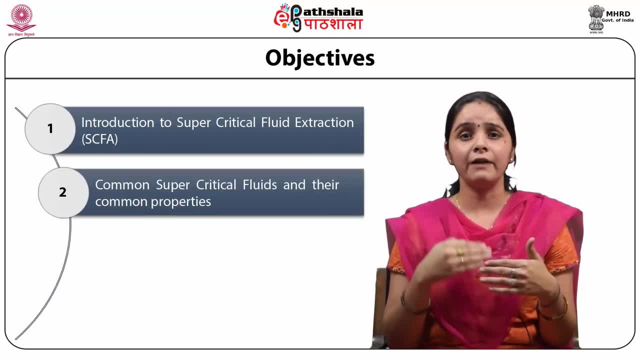 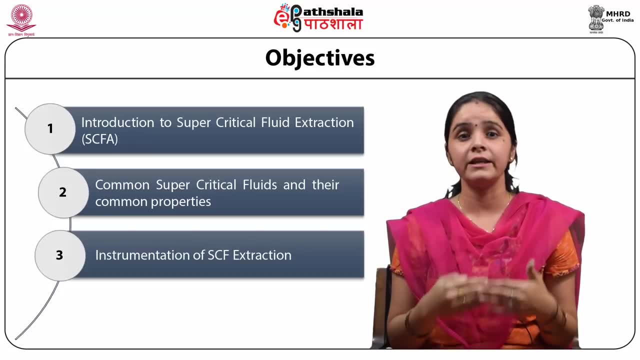 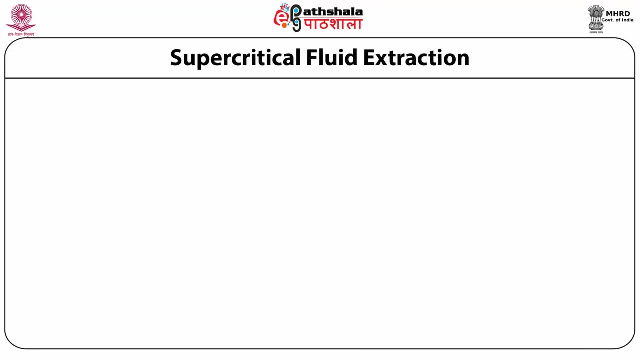 familiar with the common supercritical flutes and what are their common properties regarding instrumentation of supercritical flute extraction, its advantages and application in the extraction process. Supercritical flute extraction may be defined as separation and extraction of chemical compounds of interest from samples or products such as coffee, tea, herbs and spices, by using 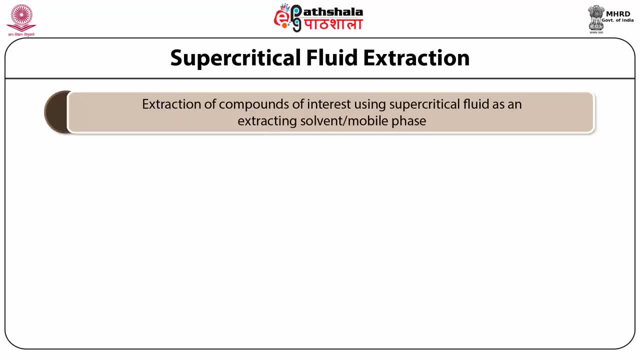 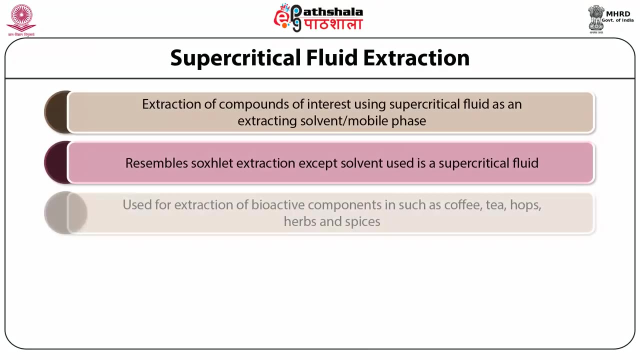 supercritical flute as an extracting solvent or mobile phase. This technique resembles solvent extraction process. Supercritical flute extraction may be defined as separation and extraction of extractions, except the fact that the solvent used here is a supercritical flute. The supercritical flute state occurs when a flute is above its critical temperature and critical pressure. 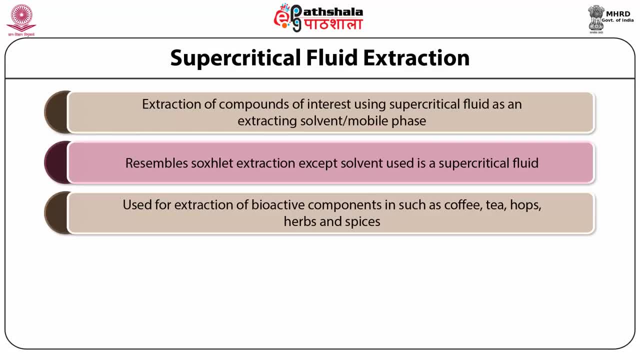 that is, between the typical gas and liquid state, during which the solvating power of mobile phase will be at its peak. The first reported observation on the occurrence of supercritical phase was made by Barron in 1822.. In 1970,. 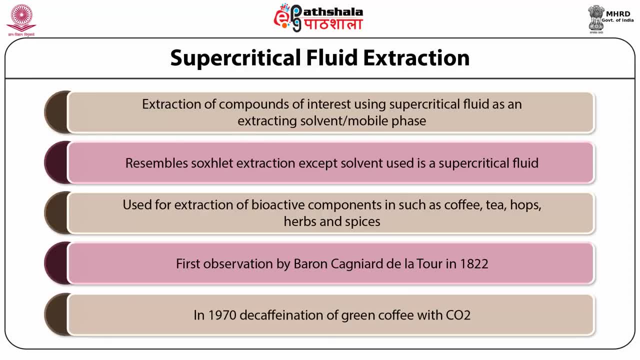 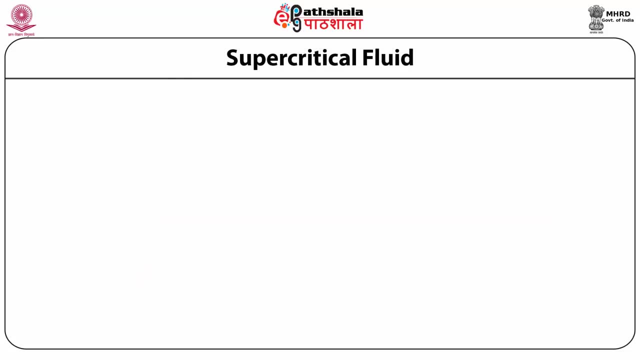 a significant development in the field of supercritical flute extraction occurred by decaffeination of green coffee with carbon dioxide as supercritical flute. What are critical flute extraction methods? Supercritical flute extraction may be defined as separation and extraction of chemical compounds of the rich phosphorus. The first reported observation on the occurrence of supercritical fluid is that the composition of a supercritical fluid in a flue can be found in the floating fluid layer in a similar form of water. talk of this as a supercritical solution, while the second part of this observation will be defined as separation of liquid and solid from the flower. The first further observation was made by Hank Johnson in 1826.. The first observation was made by Hank Johnson in 1827.. The first next search was made by Bosley and F flees of England. The first second search was made by Buck and海. The answer is. 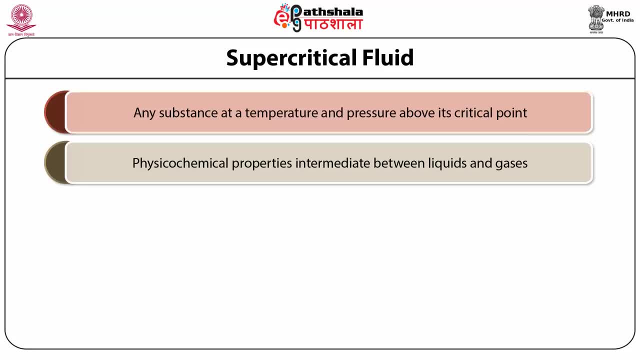 that flutes are not a liquid but a double-bee entsteations in the form of water. A supercritical fluid is any substance at a temperature and pressure above its critical point. It exhibits physicochemical properties that are intermediate between those of liquid and gases. These flutes can 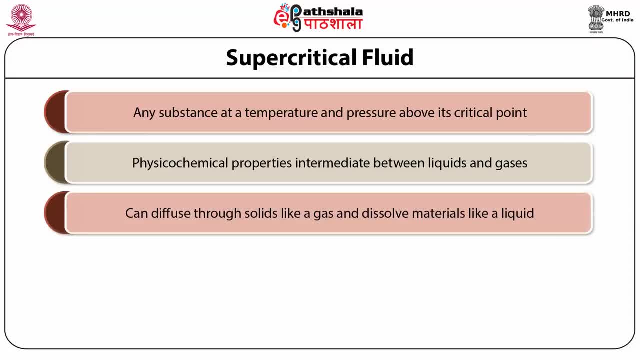 can diffuse through solid like a gas and dissolve material like a liquid. Additionally, close to the critical point, small changes in pressure or temperature results in greater changes in density, allowing many properties of supercritical fluid to be fine-tuned, Thus supercritical. 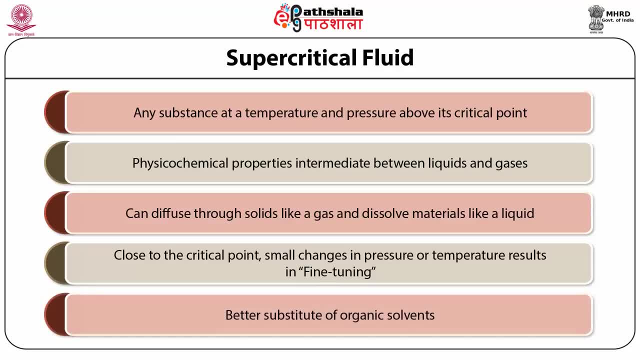 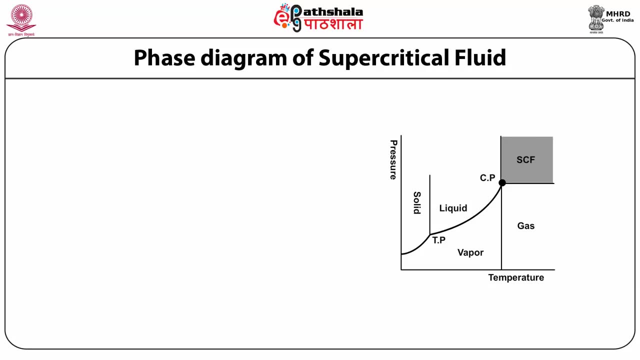 fluid can preferably substitute organic solvents for many of the industrial and laboratory processes. Phase Diagram of Supercritical Fluid. The phase diagram of supercritical fluid describes critical temperature, critical pressure and triple point. Critical temperature is the highest temperature at which a gas is produced. 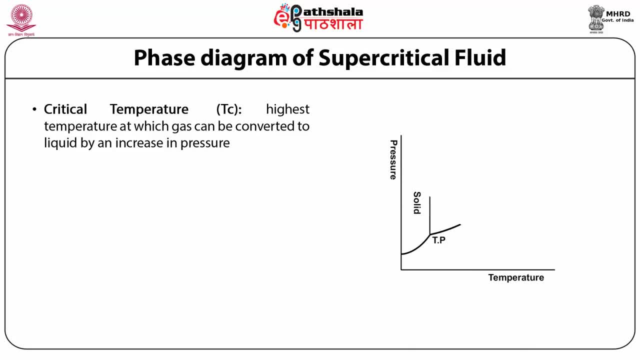 and can be converted to a liquid by increase in pressure. Critical pressure: it is the highest pressure at which a liquid can be converted to a traditional gas by increase in temperature. Triple point: it is a point at which gas, liquid and solid phases exist. 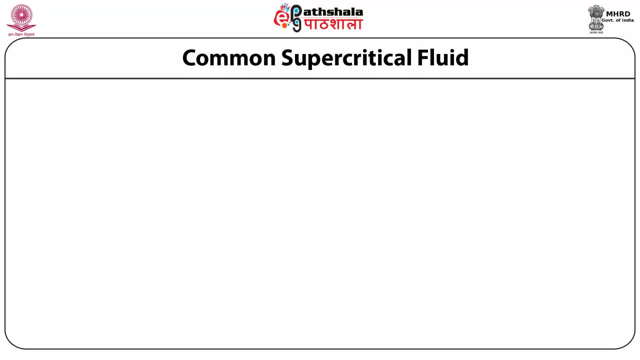 in equilibrium Common Supercritical Fluid. Among the range of supercritical fluids used, water is used for power generation and carbon dioxide for decaffeination. Apart from the fact that carbon dioxide is environmentally friendly and generally recognized as safe by the food and drugs industry, carbon dioxide is also used for decaffeination. Carbon. 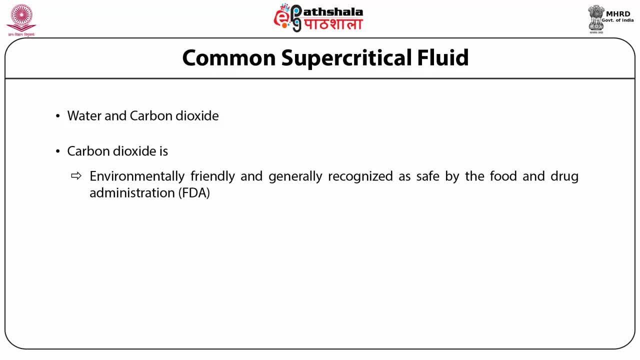 dioxide is also used in pharmaceuticals, nutraceuticals and food application. It is believed to be a good solvent because it is orderless, non-toxic, non-flammable, inexpensive, easy to remove from the product, and its critical temperature and pressure are very high. Carbon. 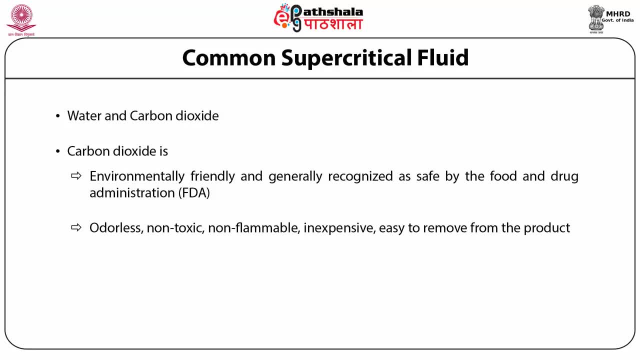 dioxide and must not be wells or hydrochloric acid based surfactants, Which are the organic and chemical components. The hydrochloric acid is looked for in water solvents and Andrew C Jackson's biochemistry theory purifies lavafeld. 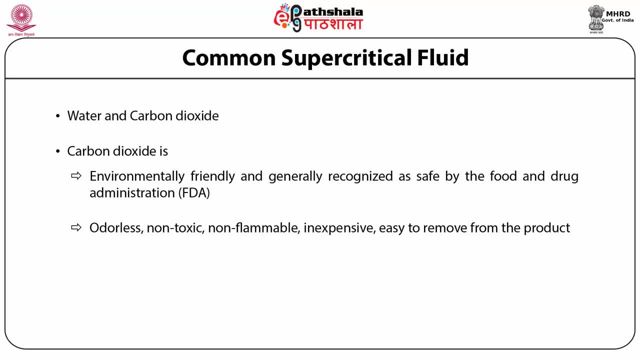 The ranking of water-based Technical Solving Equipment in roads by ranked CO2uy Alнаружi �� nein at choke al Spun side as mobile phase even allow the extraction of thermally labile, easily oxidizable compounds even at low temperatures and non-oxidant medium. 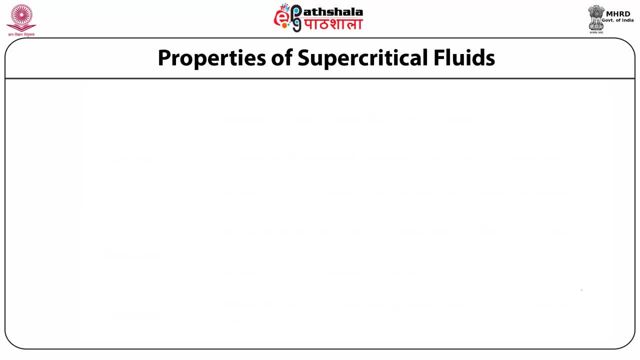 Properties of supercritical fluids. Supercritical fluids have highly compressed gases that have both liquid-like and gas-like characteristics that make them unique for chemical separation. Following are the properties of supercritical fluid. First is density. Density characteristic of supercritical fluid is between that of a gas and a liquid. but 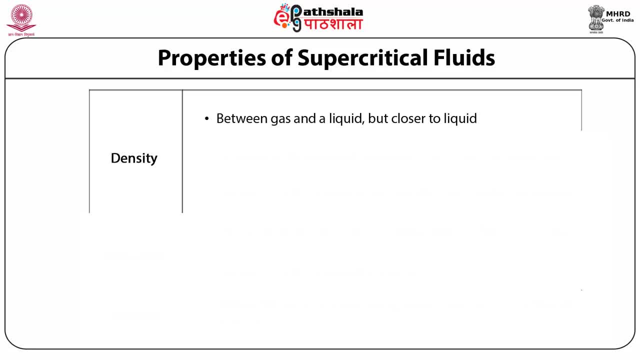 closer to liquid In the supercritical region. density increases and density decreases With increased pressure. at constant temperature, And when pressure is constant, density decreases with increase in temperature. The dissolving effect of supercritical fluid is dependent on the density value. therefore, 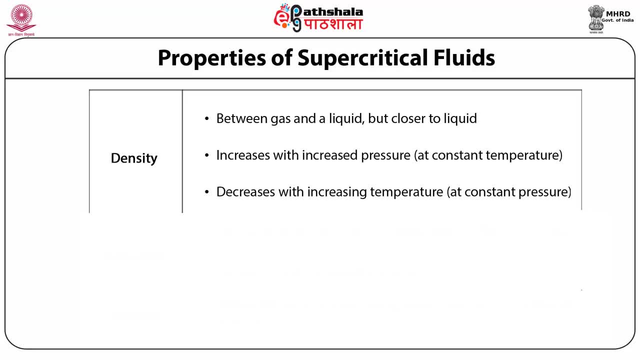 it is an essential parameter. Second property is diffusivity. Diffusivity of supercritical fluid Can be 100 times more than that of a liquid and 1 by 1000 to 1 by 10,000 times less than that of a gas. 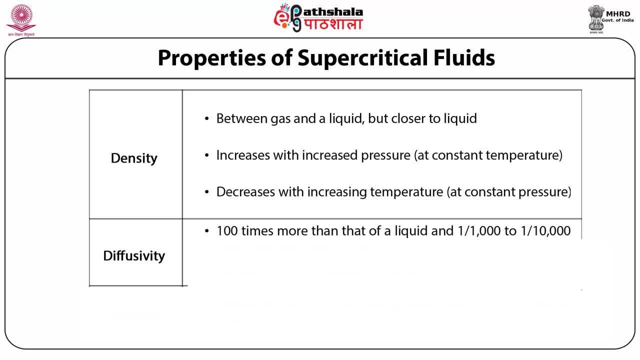 Because supercritical fluids have more diffusivity than a liquid. it stands to the reason that a solute can show better diffusivity in a supercritical fluid than in liquid. 3. Diffusivity of liquid. Diffusivity is parallel with temperature and contrary with pressure. 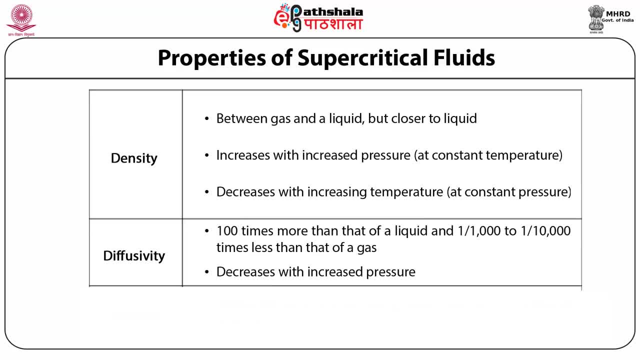 Increasing pressure affects supercritical fluid molecule to become closer and decrease diffusivity in the material. The third property is viscosity. Viscosity for supercritical fluid is almost the same as a gas, being approximately 1 tenth of that a liquid. Thus supercritical fluids are less resistant than liquid towards components flowing through. 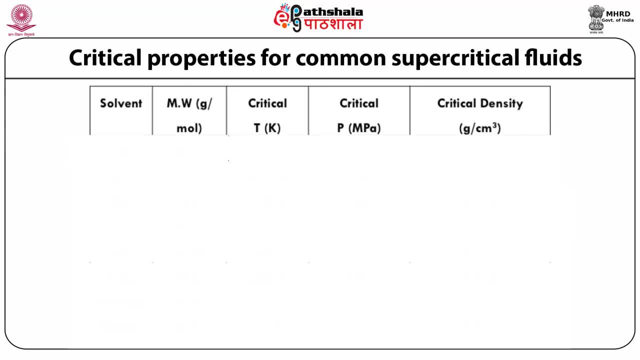 Critical properties for some components commonly used at supercritical fluids are: 1. Carbon dioxide, that is very commonly used as a supercritical fluid. its molecular weight 44.. 2. Critical density in Kelvin is 304.1. 3. Critical pressure in MPa is 7.38. 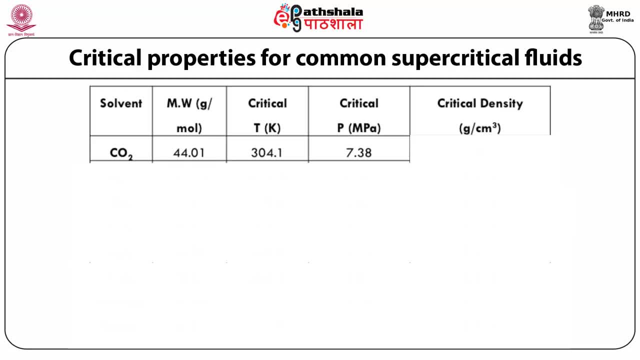 4. Critical density in g per cm3 is 0.469. 5.. The next most common used solvent is water with critical temperature 647.096 Kelvin, critical pressure 22.064 and critical density 0.106 Kelvin 6.. 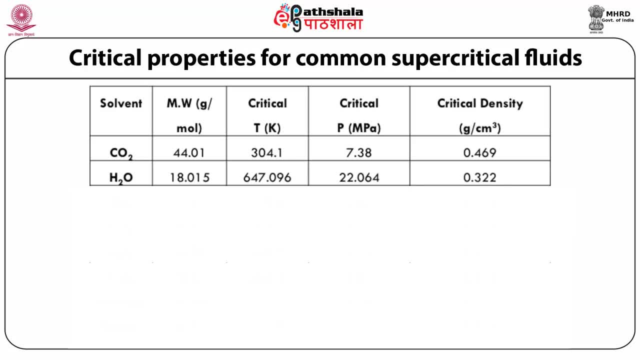 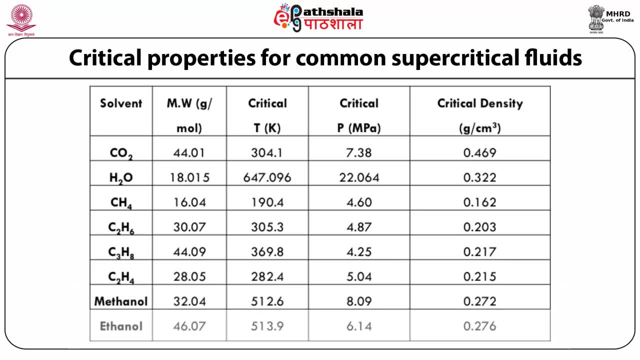 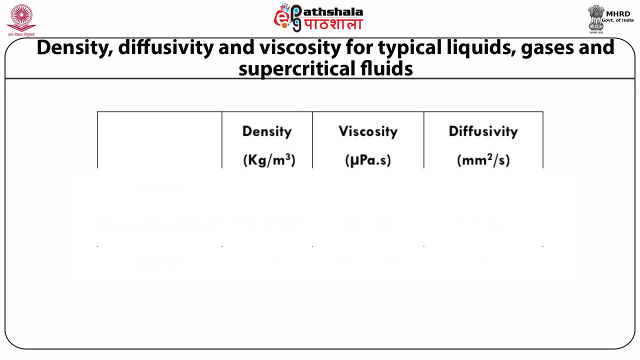 Diffusivity of liquid. Other solvents used are methane, ethane, propane, methanol and ethanol. The following table shows the density, diffusivity and viscosity for typical liquids, gases and supercritical fluid. Compared to the gases, the supercritical fluids have higher density, higher viscosity and. 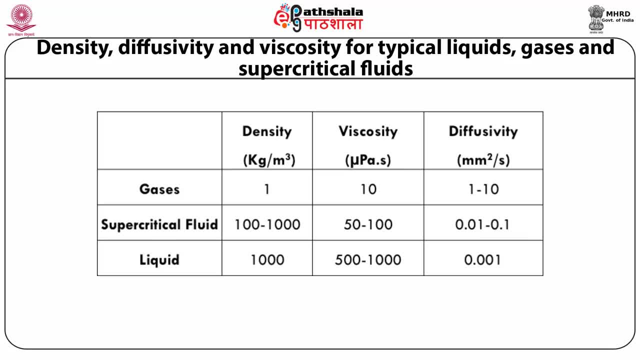 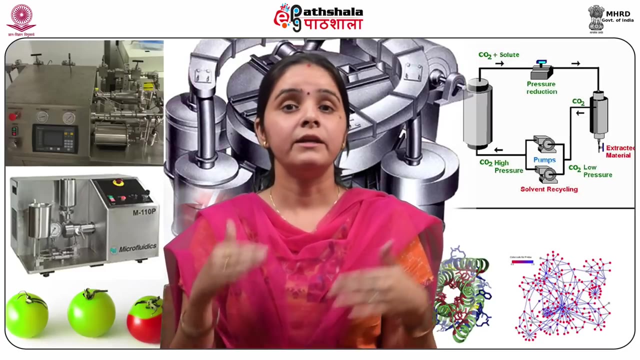 lower diffusivity. Compared to liquid, the supercritical fluid has density closer to liquid, viscosity lower than liquid, and diffusivity is higher than liquid. The Solvating Power of Supercritical Fluids. The solvating power of supercritical fluids. 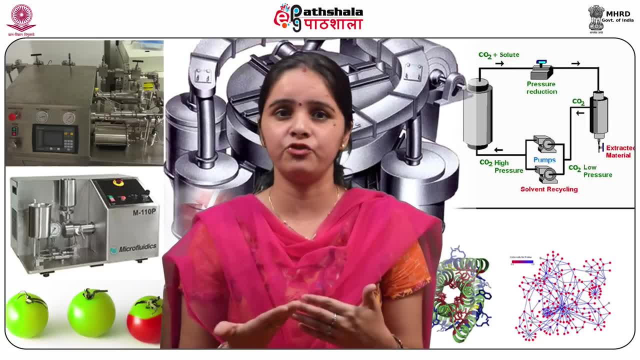 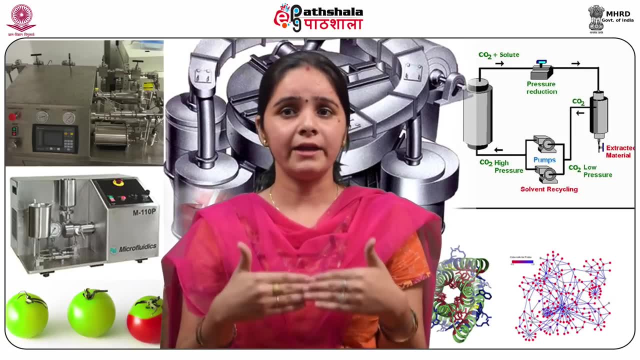 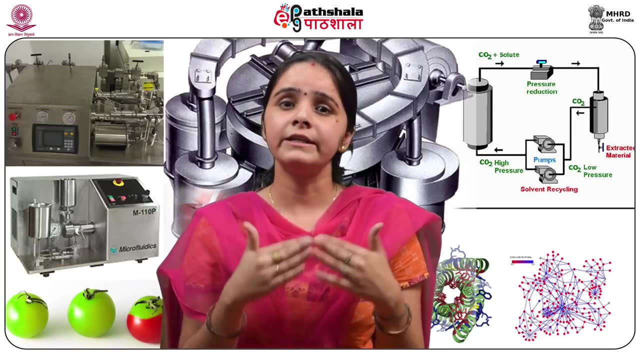 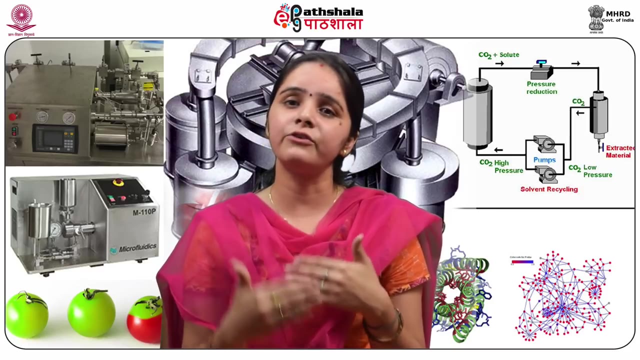 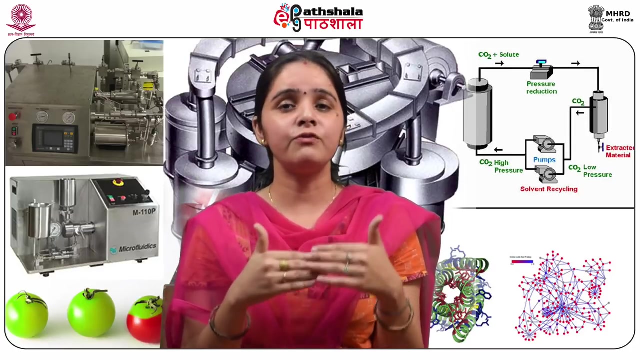 roots ultimately defines their limit of application, because the solubility of analyte typically increases with density and maximum rate of increase in solubility with pressure is generally observed near the critical pressure, where the rate of increase in density with pressure is greatest. Hence there is often a linear relationship at constant temperature between 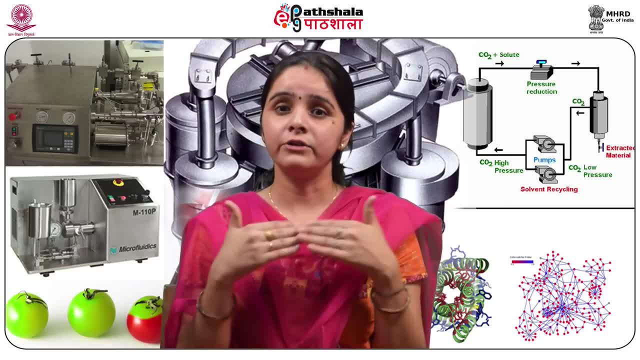 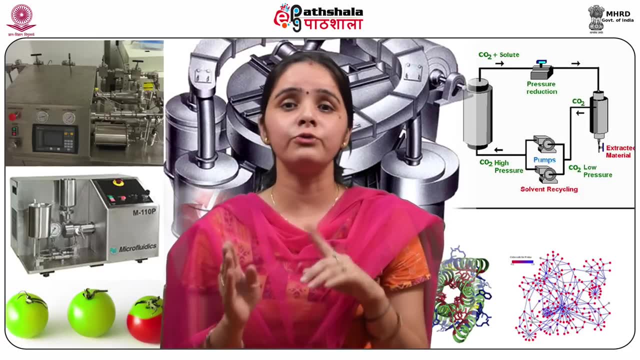 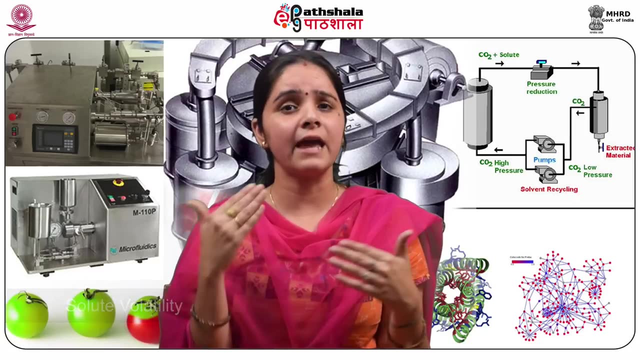 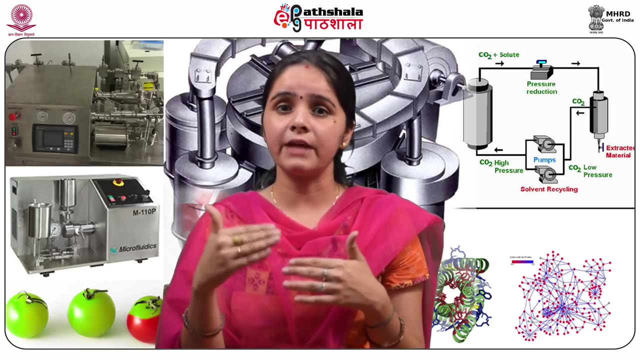 solubility and fluid density for dilute solutions of non-volatile compounds up to the concentration where solute-solute interaction become important At constant pressure, when solute volatility is extremely low and at density less than or near the critical density. increase in temperature will typically decrease the solubility. However, the solute 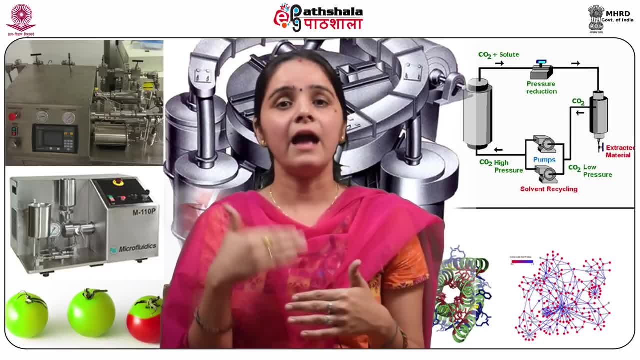 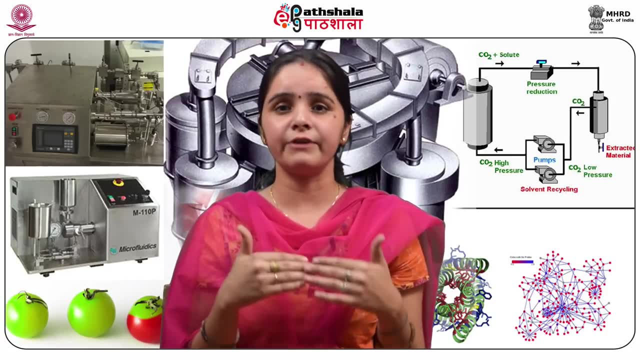 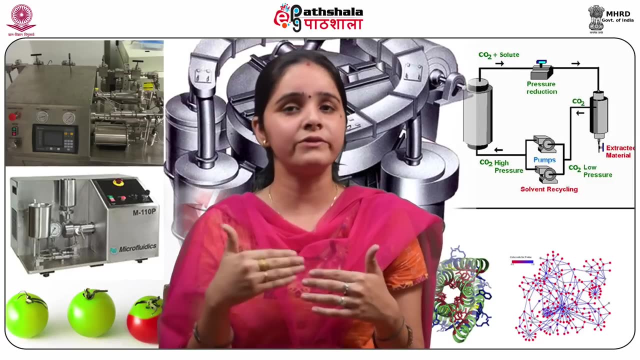 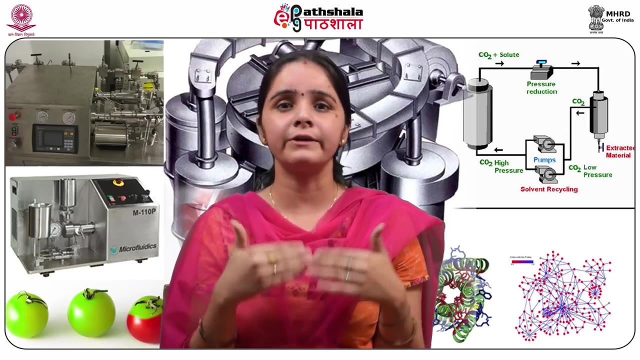 entrainment in the fluid may increase at sufficiently high temperature where solute vapor pressure also becomes significant. Under conditions of constant density, solubility generally increases with temperature. The polar solutes are the most important solute and most soluble in the polar supercritical flutes, Although nominally the non-polar flutes. 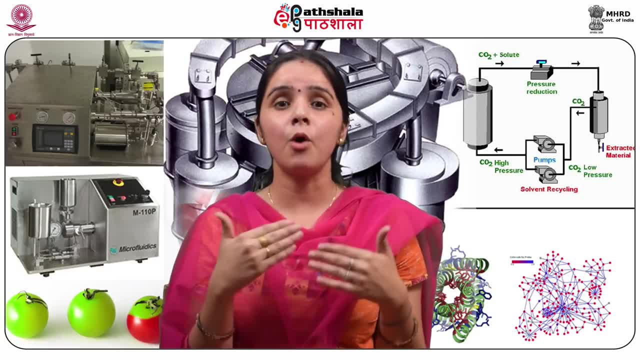 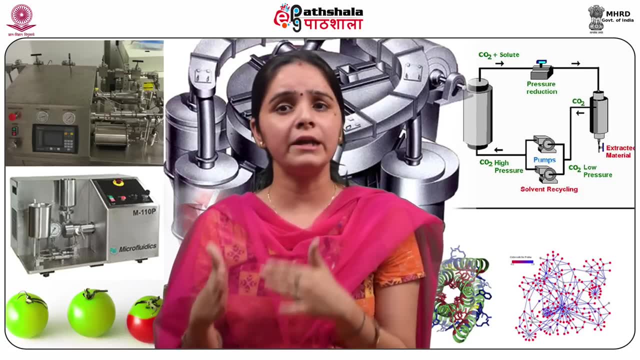 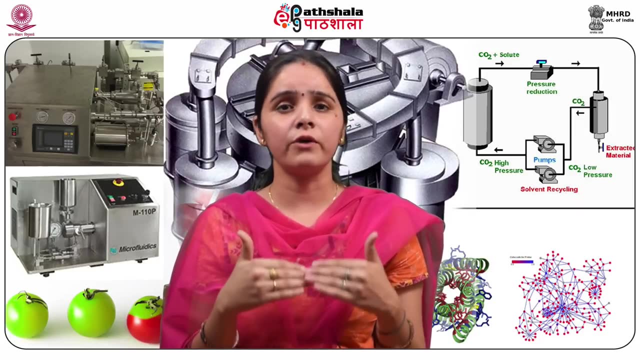 can be remarkable. good solvent for many moderately polar compounds. The supercritical flutes have solvating power, the similar to the liquid organic solvent, but advantages are they have higher diffusivity, lower viscosity and the lower surface tension Since the solvating. 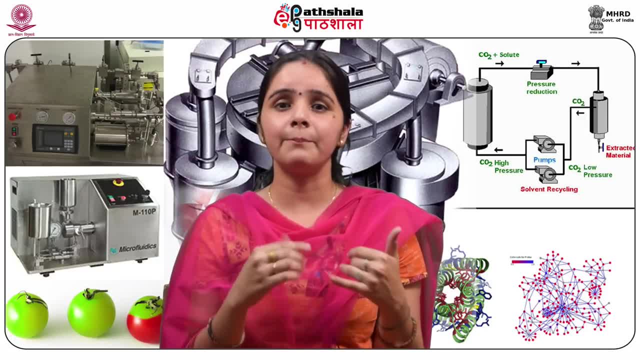 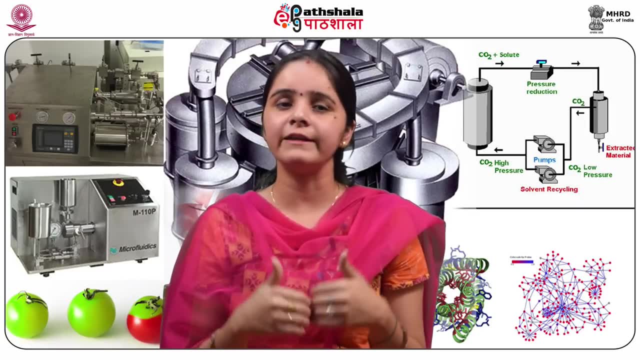 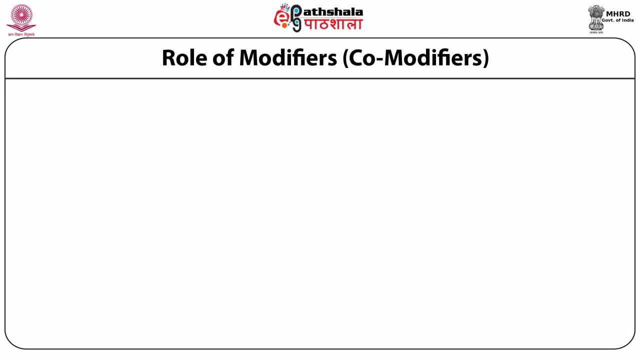 power can be adjusted by the changing pressure and the temperature. the separation of analyte from supercritical flutes solvent is very fast and easy. Role of modifiers or co-solvents: In many cases slow solute extraction kinetics or limiting analyte solubility in the flutes. 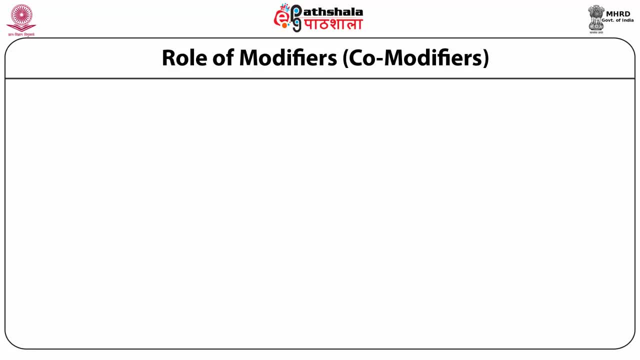 phase can be overcome by the addition of modifiers or co-solvents to the supercritical flutes phase. By adding modifiers to a supercritical flutes, like methanol to carbon dioxide, the polarity can be changed for having more selective separation power. The co-solvent interacts strongly with the 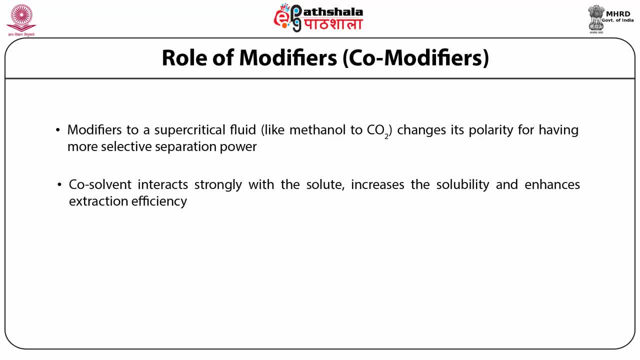 solute significantly increases the solubility solubility and enhances extraction efficiency. For example, addition of 1-10% of methanol or ethanol to carbon dioxide expands its extraction range to include more polar lipids, and addition of 9% methanol increases the solubility of cholesterol by 100 fold. 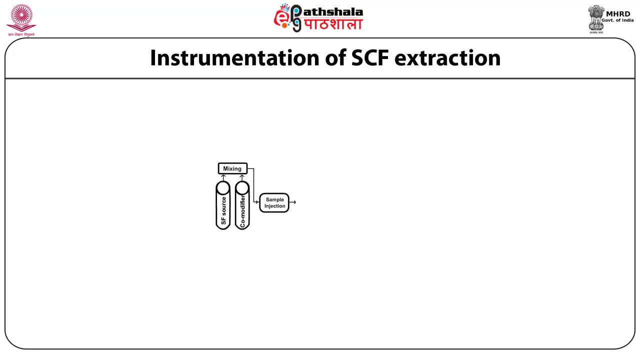 Instrumentation of supercritical fluid extraction In the instrumentation from a fluid source, commonly tanks of carbon dioxide and co-modifiers. both are mixed with sample and injected into extraction cell through syringe pump having a pressure rating of at least 400 atm. The liquid is. 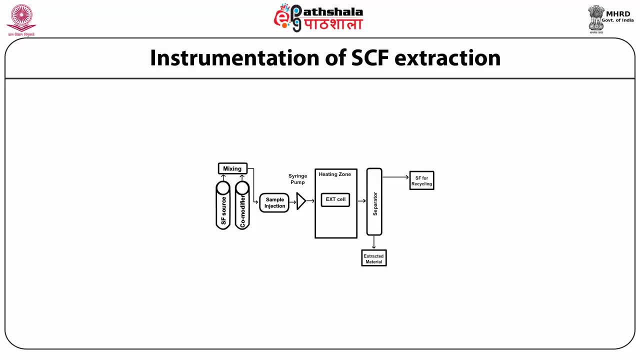 pumped to a heating zone, where it is heated to supercritical condition. It then passes into the extraction vessel, where it rapidly diffuses into solid matrix and dissolves the material to be extracted. The material is swept from the extraction cell into a separator at lower pressure and the 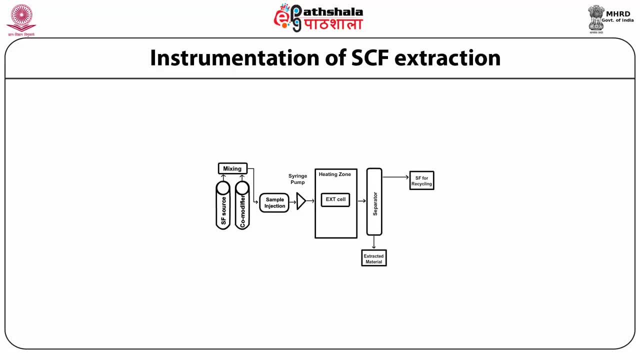 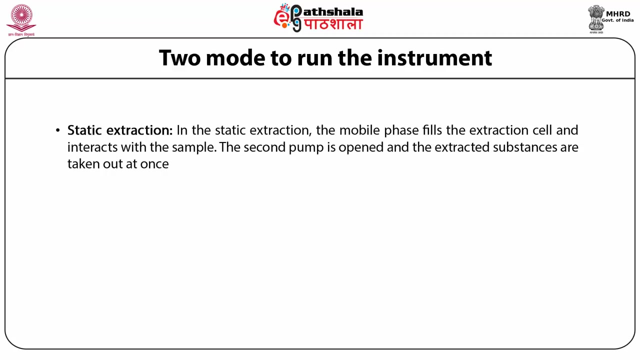 extracted material settles out. The carbon dioxide or other supercritical fluid can then be cooled, recompressed and recycled, or discharged to atmosphere Mode to run the instrument. There are two principal modes to run the instrument. The first is static extraction. In the static extraction there are two distinct steps in 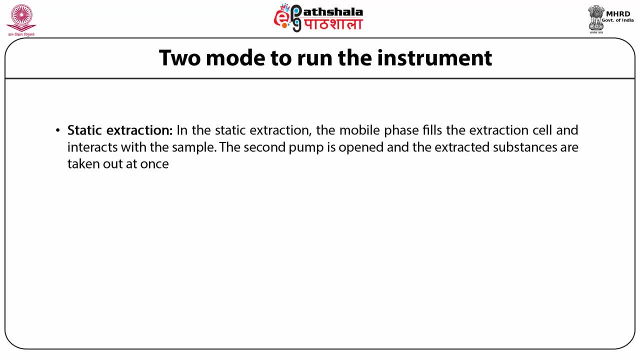 the process. First the mobile phase: 2., 3., 4., 5., 6., 7., 8., 9., 10., 11., 12., 13., 14., 15.. 16., 17., 18., 19., 20., 21., 22., 22., 23., 23., 24., 24., 25., 26., 27., 28., 29.. 30., 31., 32., 33., 34., 34., 35., 36., 37., 38., 39., 39., 40., 41., 42., 42., 43.. 43., 44., 44., 44., 45., 46., 46., 47., 47., 48., 49., 49., 50., 61., 82., 83., 84.. 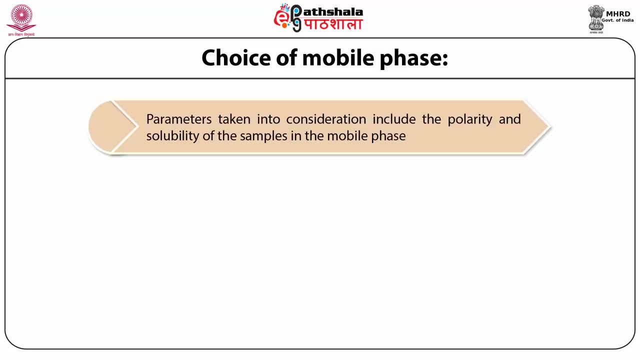 85., 86., 87., 80., 69., 81., 82., 69., 63.. polarity and solubility of the samples in the mobile phase. Carbon dioxide is the most common mobile phase for supercritical fruit extraction. 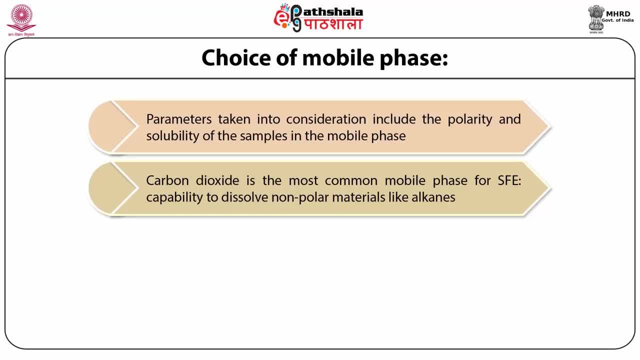 It has a capability to dissolve non-polar materials like alkanes. For semi-polar compounds such as polycyclic aromatic hydrocarbons, aldehydes, esters, alcohol, carbon dioxide can be used as a single component: mobile phase. 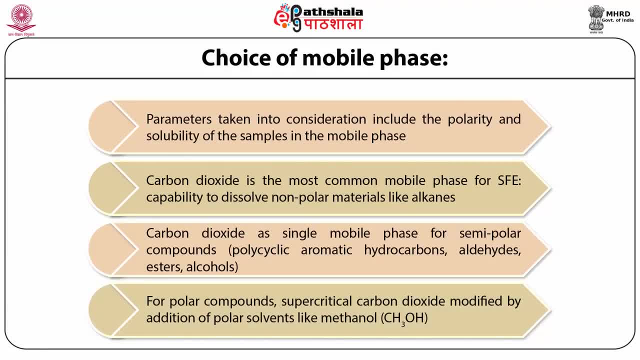 However, for compounds which have polar characteristics, supercritical carbon dioxide can be used as a single component. Carbon dioxide must be modified by addition of polar solvents like methanol. These extra solvents can be introduced into the system through a separate injection pump. 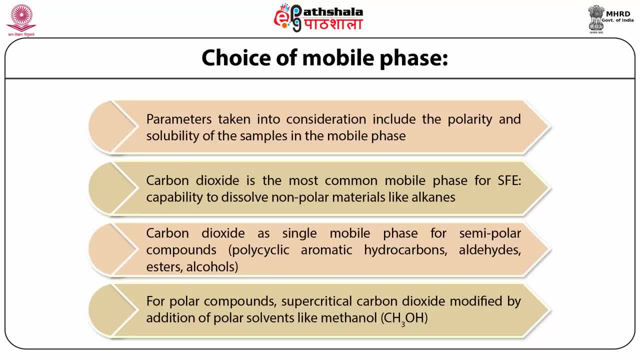 There are two main procedures to study with co-solvents or modifiers in supercritical fluid extraction. The first one is the supercritical fluid extraction. The second one is the supercritical fluid extraction. The first one is mixing of the modifier with the carbon dioxide flow, while the second 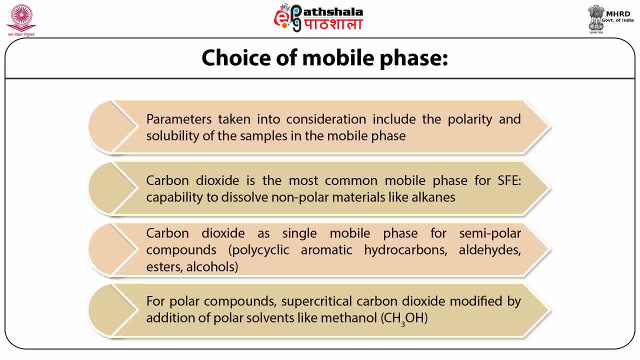 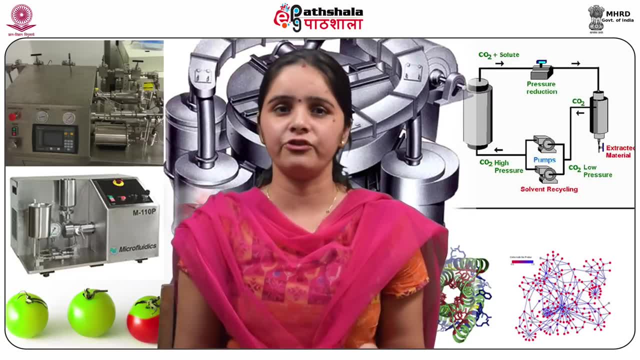 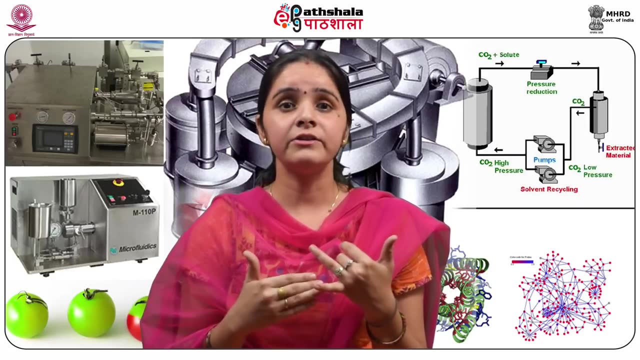 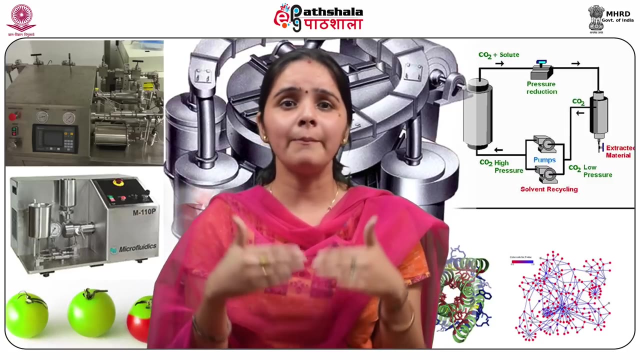 mixes the modifier with raw material in the extraction cell. Next is the advantages of supercritical fluid extraction. The foremost advantage is the supercritical fluids are cheap, inert and non-toxic in nature. The supercritical fluid can be separated from analyte by simply releasing the pressure. 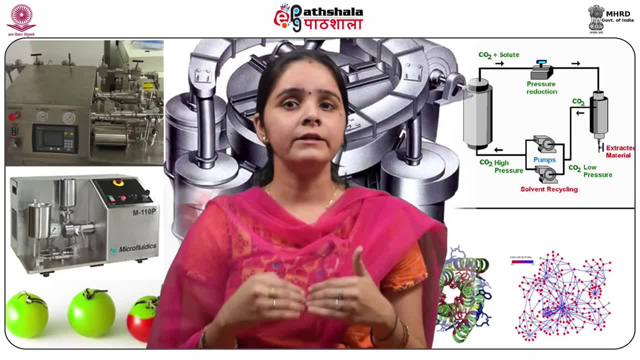 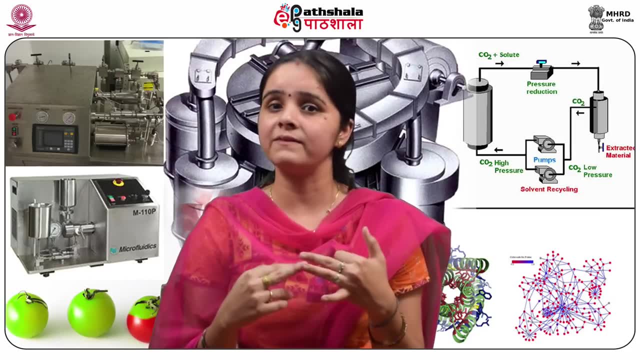 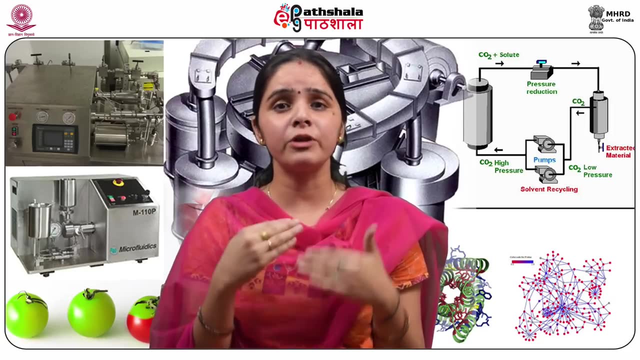 leaving almost no traces. Third, the supercritical solvents are chemically inert, harmless and inexpensive. They can be released to the atmosphere without leaving any waste. This is the most important advantage of supercritical fluid extraction. Because of this, the supercritical solvents can be released to the atmosphere without 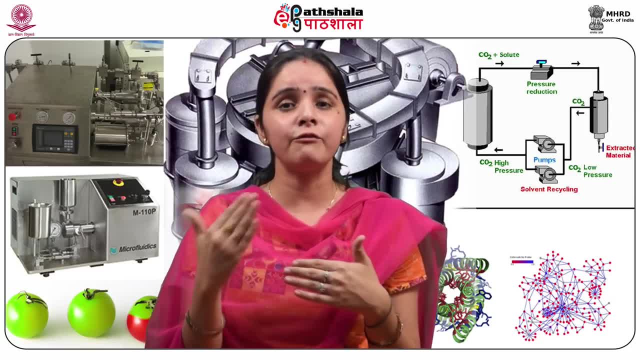 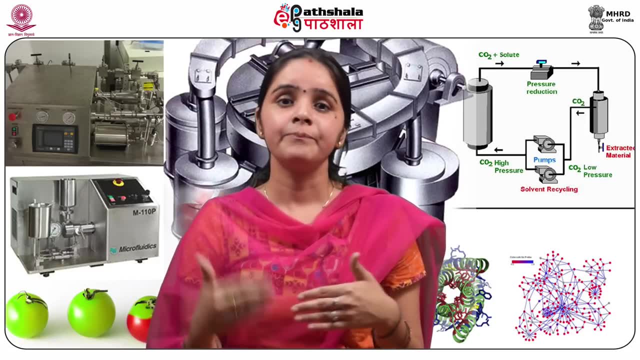 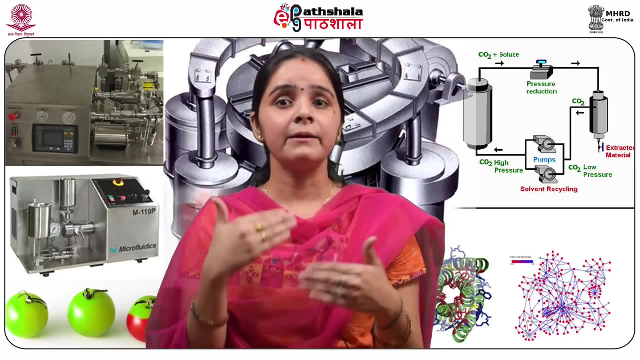 leaving any waste. The second advantage is the supercritical fluid extraction is considered as a green technology because it is environmentally friendly. The selectability of solvent in the supercritical fluid extraction: strength of solvent can be select by changing the pressure as well as the temperature. 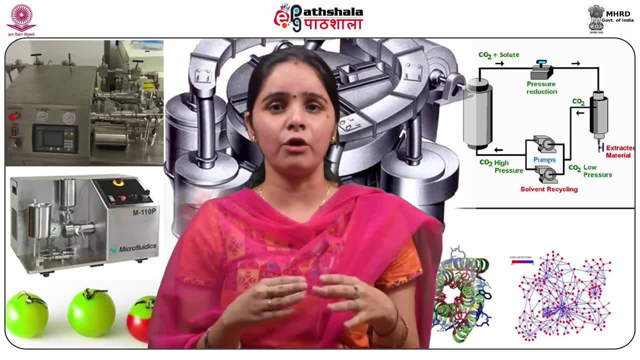 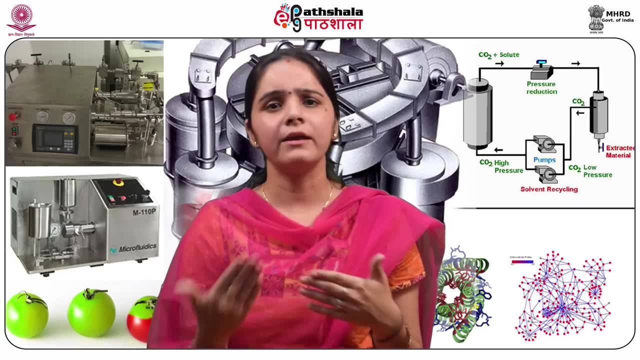 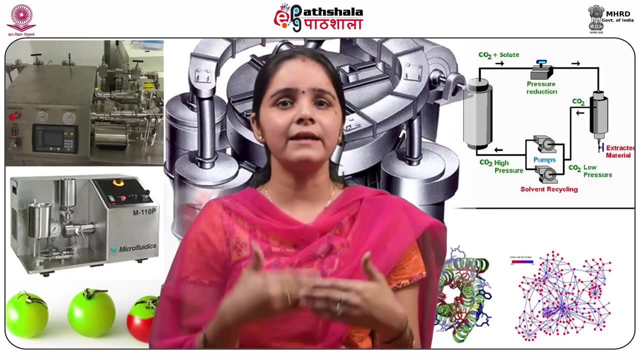 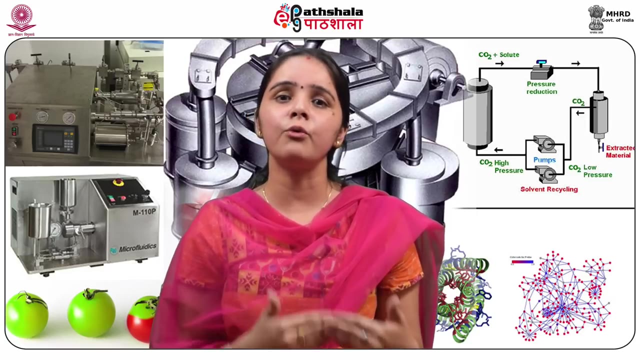 Means. if you want to increase the selectivity of solvent, you have to just change the temperature and the temperature. The supercritical fluid extraction is a very rapid process, comparable to the normal extraction process. It completes in 10 to 60 minutes. Diffusivity are much faster compared to liquids and therefore the extraction can occur faster. 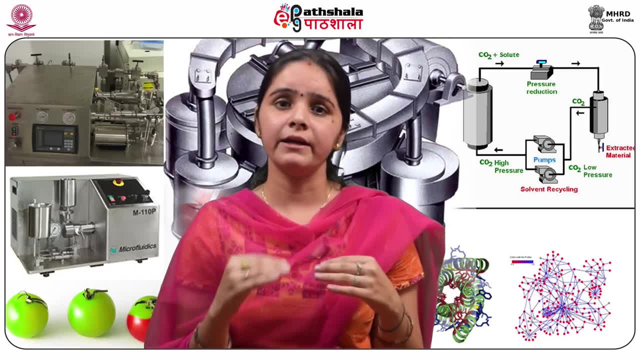 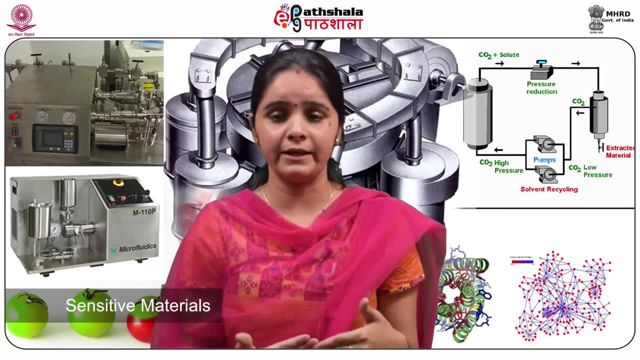 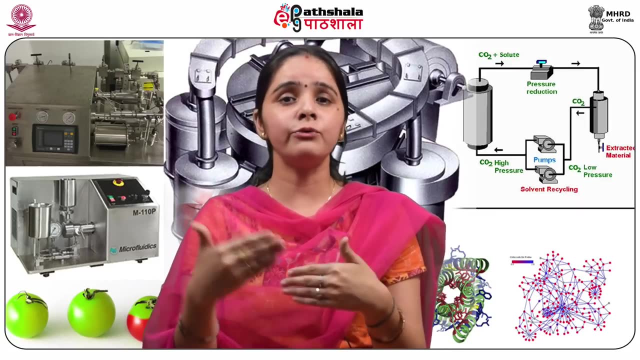 Next important advantage is there is no heating is required to get rid the extraction liquid. It is good for the temperature sensitive material Because what we have seen in the conventional extraction process, that for removing the solvent you have to heat the sample. If under vacuum you are heating, you have to go up to 60 degrees centigrade. 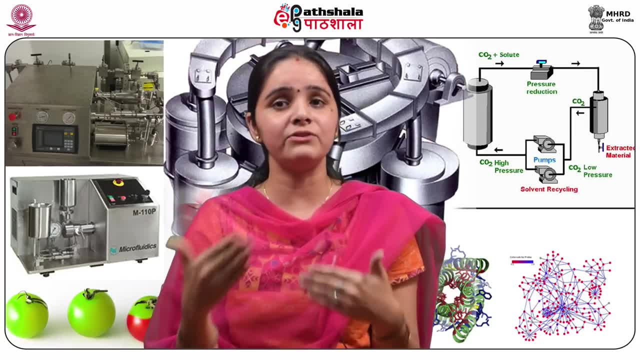 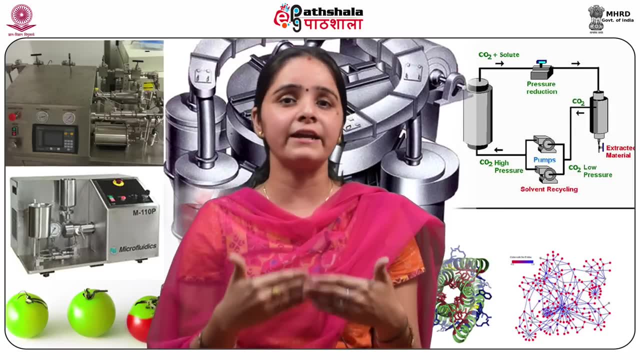 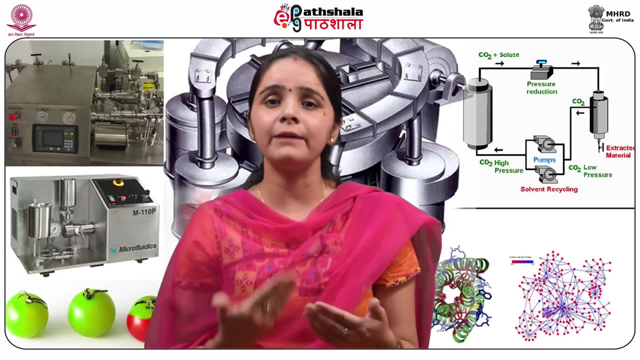 So the conventional methods are not good for the temperature sensitive material. For those temperature sensitive material, this supercritical fluid extraction technique is very good Because no heating is employed And the next year the recovery of analyte become very simple if you are using the supercritical. 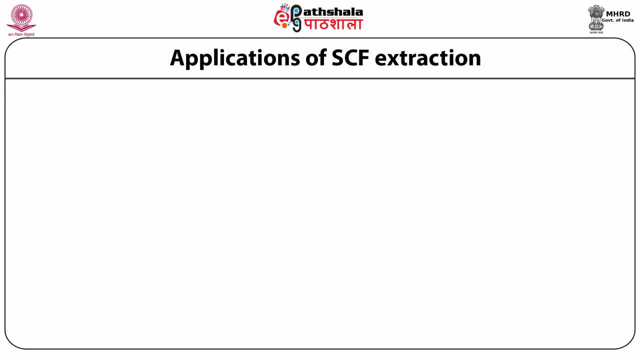 fluid extraction method. Applications of supercritical fluid extraction to food processing. The supercritical fluid extraction technology has advanced tremendously since its inception And it is a method of choice In many food industries. Over the last two decades it has been well accepted as a clean and environmentally friendly. 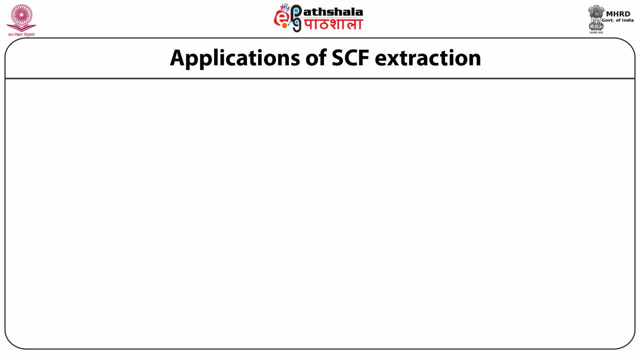 green processing technique And, in some cases, an alternative to organic solvent based extraction of natural product. Important applications are as follows. The number one is 1. The application of essential oils and its derivative for use in food, cosmetic and pharmaceutical industry. 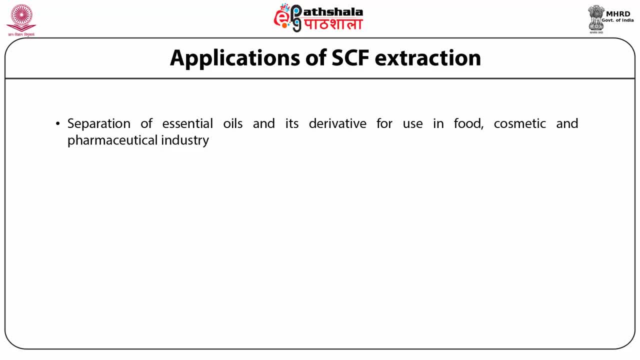 The supercritical fluid extraction has been proved in effective production of high quality essential oil compared to conventional hydro distillation. The second application is 2. Removal of fat from food. Supercritical fluid extraction is used for extraction of oil to produce fat free and. 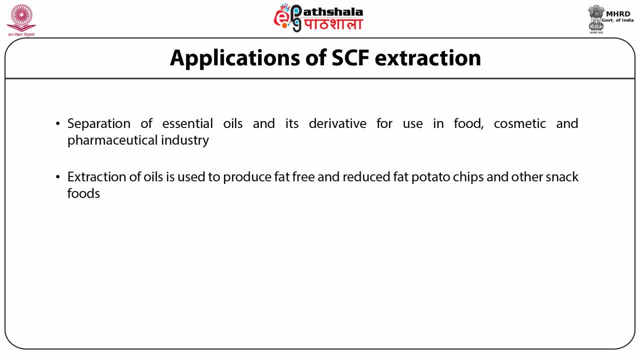 reduced fat potato chips and other snack food to satisfy the consumer need for lighter food. 3. The third application is: 4. Enrichment of vitamin E from natural sources. Supercritical fluid extraction is used in the separation of tocopherol and other antioxidants. 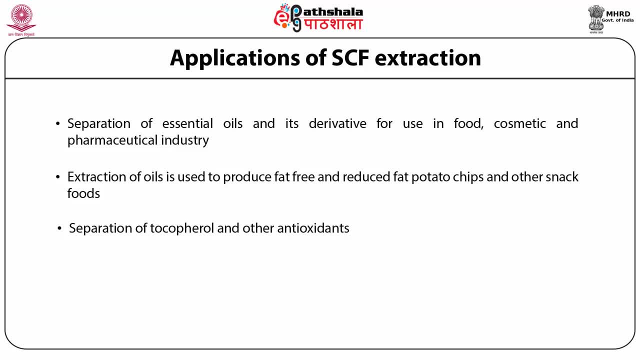 Because they have greater solubility in carbon dioxide, and it also avoids the step of vacuum distillation. 5. The second application is: 4. Removal of oil from food and other animal products, Which usually result in the thermal degradation of product. 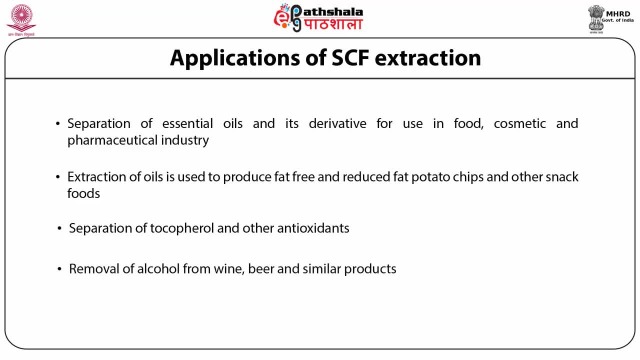 6. The supercritical fluid extraction is also used for removal of alcohol from wine or beer. It is achieved by removing ethanol from water without removing the aroma compound 7.. Next application is 8. Microspheres or large capsules can be formed with the help of supercritical fluid extraction. 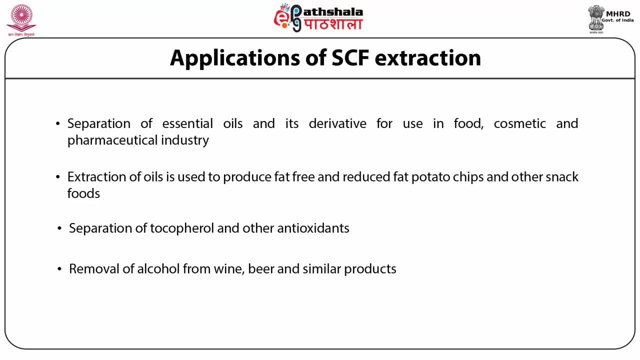 It is also used for extraction and characterization of functional compound after coupling with HPLC, for characterization of antimicrobial compounds, as well as for food preservative. It is also used in extraction of carotenoids with minimum loss of activity. The next application of supercritical fluid extraction is in the area of food safety. 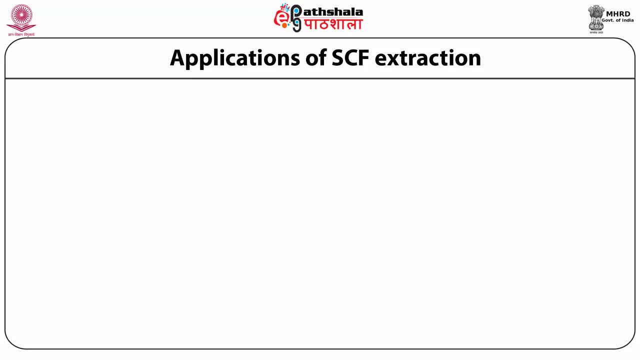 It has been used in food pollutant analysis, mainly pesticide residue pesticides, organochlorine, organophosphorus, organonitrogen, etc. and pyrethroids, as well as for other environmental pollutants. It is also used in the rapid analysis of fat content from numerous products ranging from 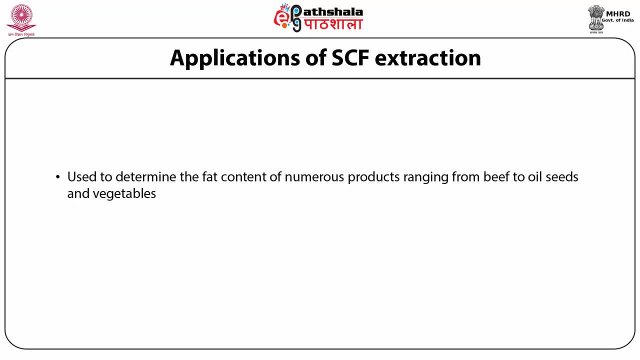 beef to oilseeds like soya bean, sunflower, safflower, cottonseed, etc. and from vegetable. The next application is in the area of decarbonization-moving compounds which are not soluble in supercritical fluids. It could be used as an anti-solvent. 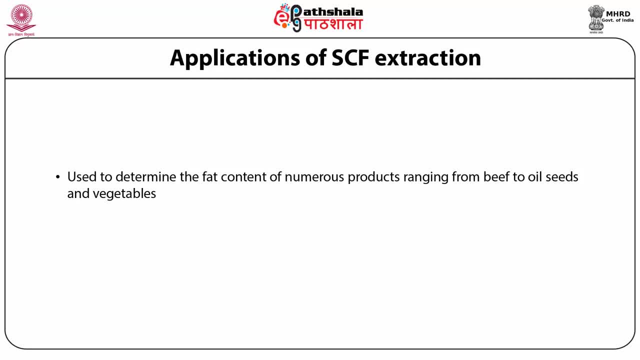 Supercritical fluid. main application is in the area of decaffeination- alkaloids- organic compounds with bitter taste and toxic effects on animals as well as on humans, but they possess the therapeutic effects when applied to animals and their animals Maintain the Pandemie and promote the HIV wave in the human body. 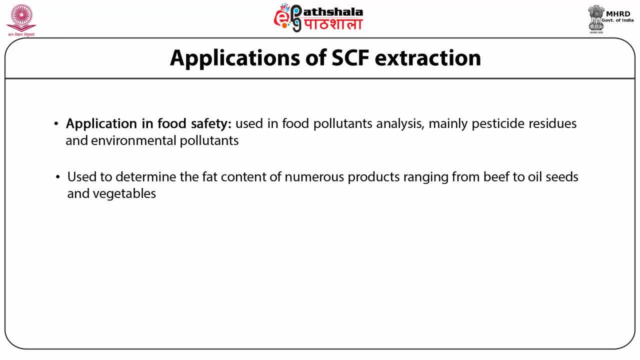 Caring to yourself and others, applied in moderate doses, are mainly found in many natural plants. Alkaloids such as caffeine, morphine, among other, are the active component in a variety of stimulants and medicinal products, and their recovery from natural plant is of great interest to the food pharmaceutical. 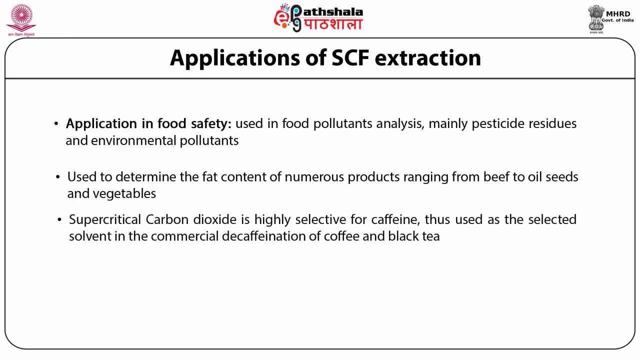 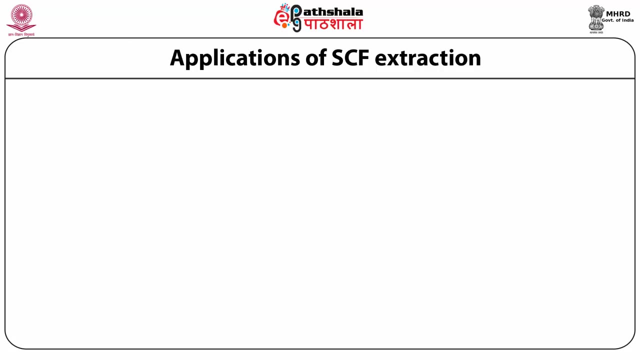 and cosmetic industry. Supercritical carbon dioxide proved to be highly effective for caffeine extraction because of selected solvent and commercially used in decaffeination of coffee and black tea. Supercritical fluid extraction is also used in denicotinization of tobacco means for production of tar free tobacco. It is also important in chiral separation. 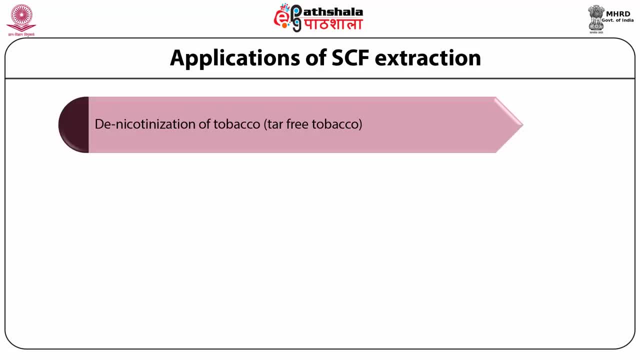 that is a very important issue for pharmaceutical industry. The solvent and anti-solvent properties of supercritical fluid is also used in the recovery of alkaloid such as theophylline and theobromine. It is used for the microbial inactivation of foods and its implementation. 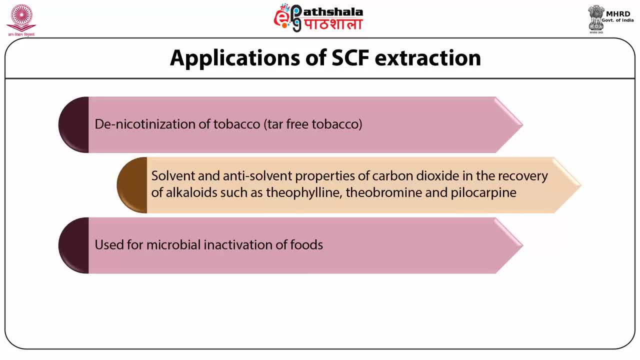 as an innovative technique for the sterilization of thermally and pressure sensitive material, is gaining popularity nowadays. Supercritical fluid extraction is used for reduction of cholesterol from dairy and food product because cholesterol is soluble in supercritical carbon dioxide and even more in supercritical ethane. 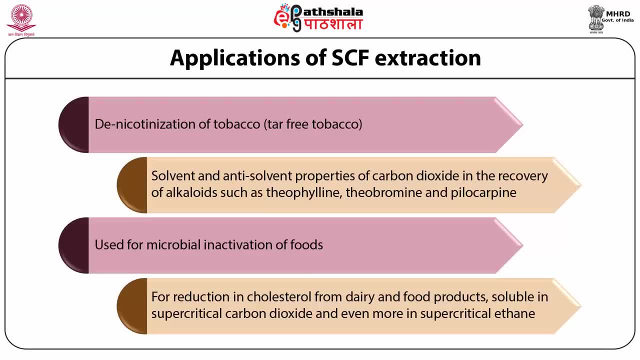 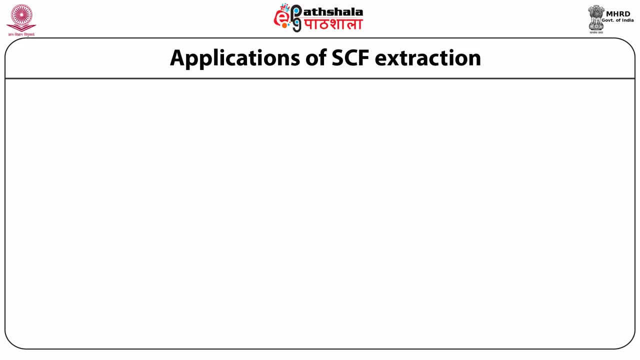 The cholesterol high related to high blood. cholesterol level in the blood is related to heart diseases and cancer. The next area of supercritical fluid extraction application is it has been proved effective for the production of high quality cocoa butter from cocoa bean. It is used in the production of particulate products. 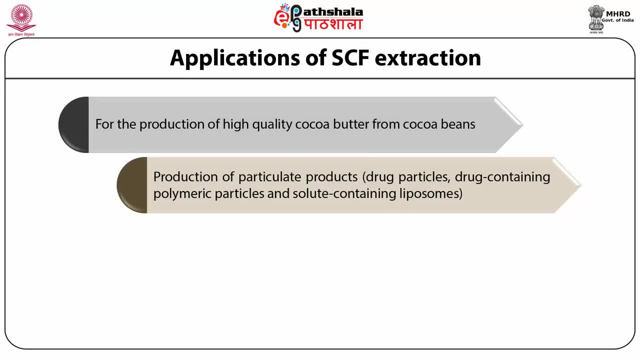 like drug particles, drug containing polymeric particles and solute containing liposome. Supercritical water oxidation is an environmentally attractive technology through which the organic material is produced Can be oxidized to carbon dioxide, water and gaseous nitrogen. It is one of the new potential. 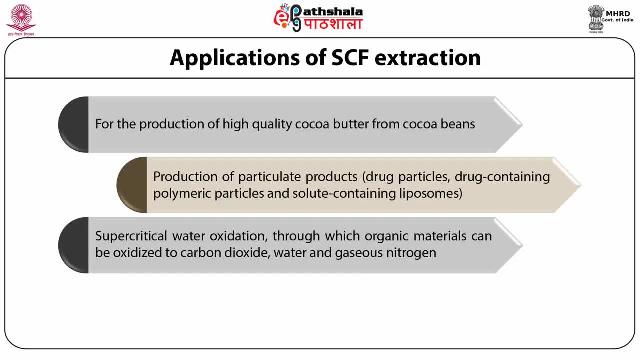 application of supercritical fluid technology. In addition to the homogenization of reaction mixture, the high oxygen concentration are attained in supercritical water. The application of supercritical water for the safe detection and destruction of toxic material is a viable alternative to incineration and land disposal. 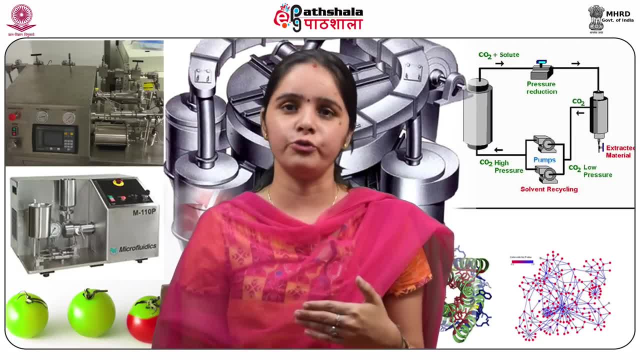 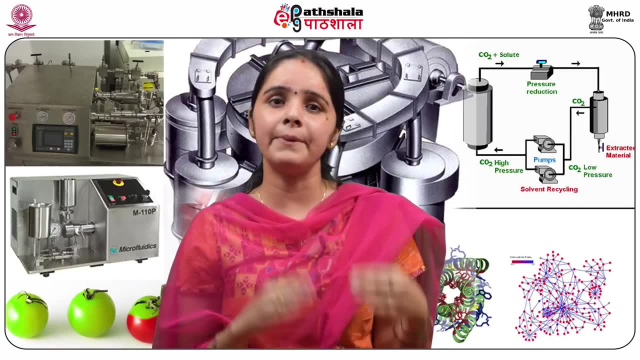 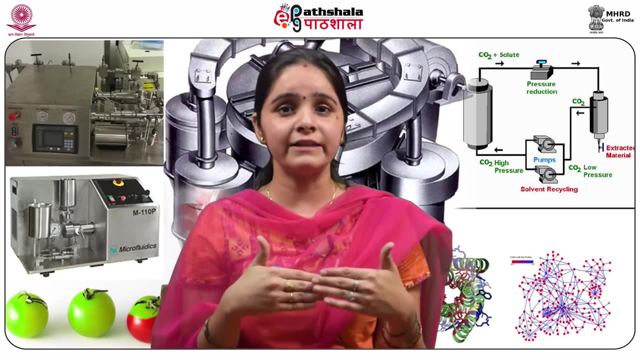 Students. now we have come to the conclusion part of this module. So here we have seen that supercritical fluid extraction is a better technique compared to the conventional technique. They it has because several advantages, and the most important advantages is that it can be used in precise extraction process. 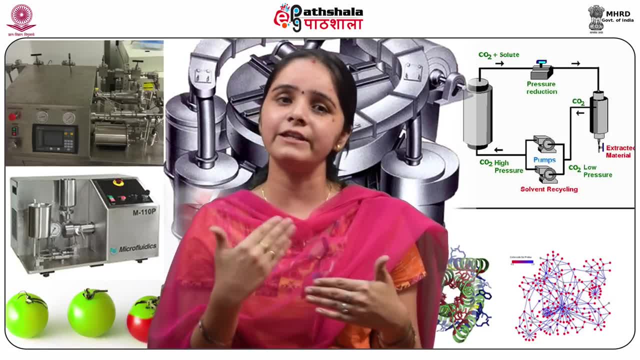 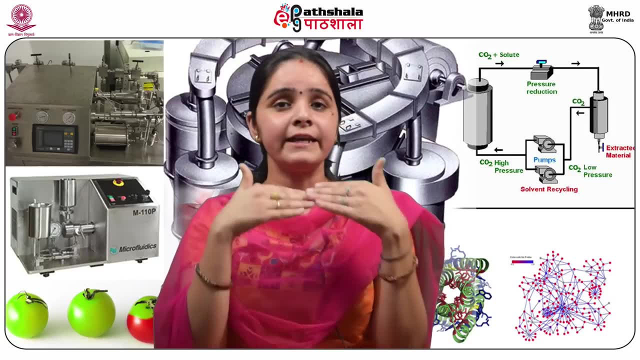 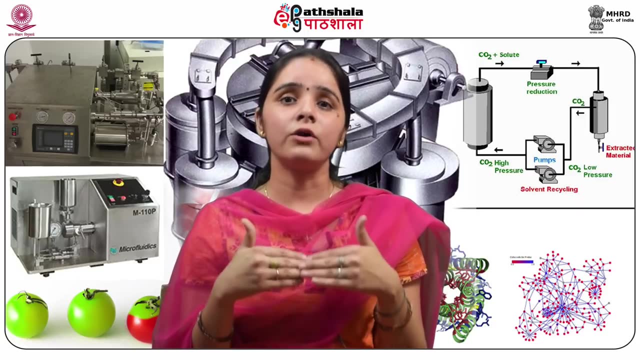 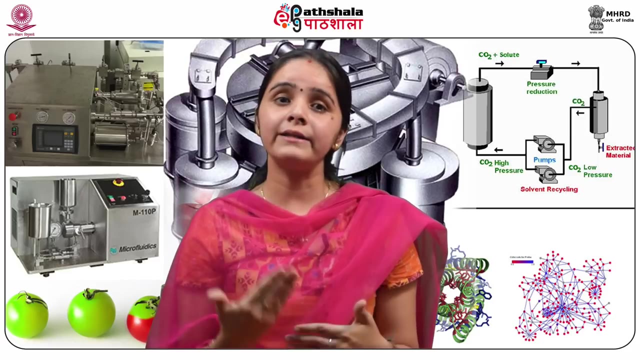 is that it can be employed for heat sensitive ingredient. next is the choice of solvent in super critical fluid extraction. we have seen that there are different solvent that can be used for the super critical fluid extraction, but the carbon dioxide is the important one because its critical temperature and pressure is low, so it can be employed for the extraction of heat sensitive. 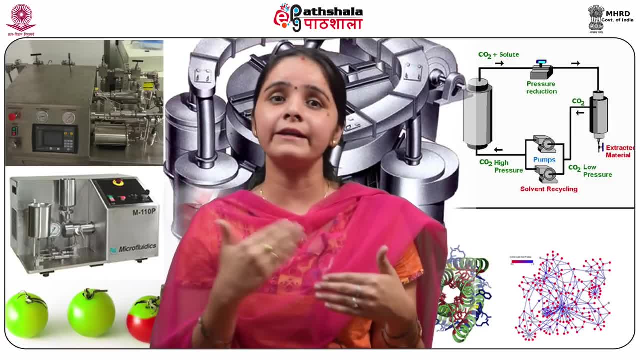 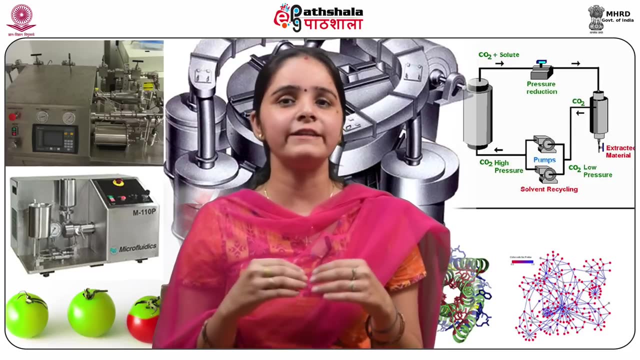 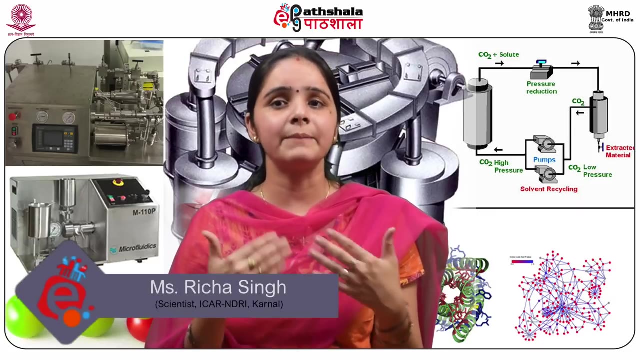 ingredient. important advantage of super critical fluid extraction was green technology means it is very safe for the environment and now there is a tendency to use the environment friendly solvents, so this technique is a replacement of conventional technique. the next advantage was that it was the safe destruction method for the toxic material and it can be used as a viable alternative. 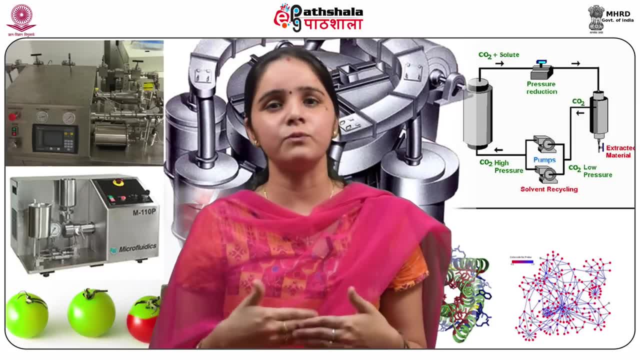 for the insecticide irrigation and as well as for the length disposal. thank you, 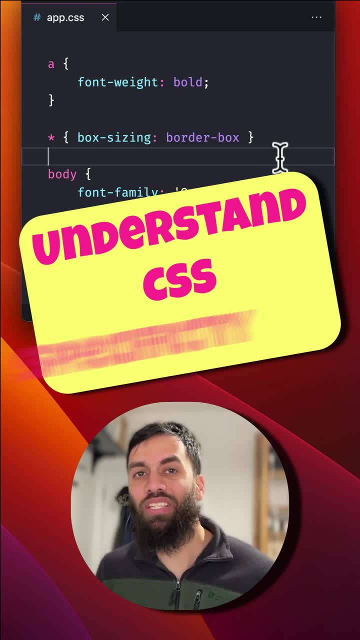 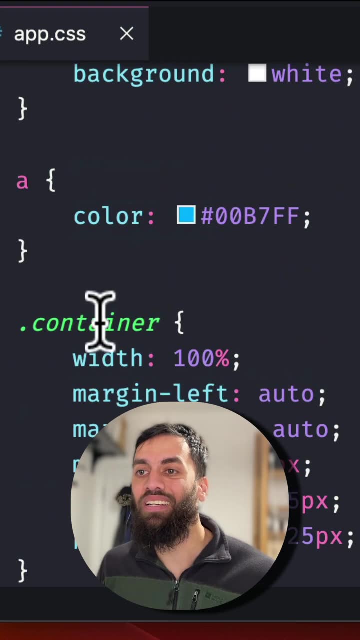 Part of being a good web developer involves understanding the basics of selector specificity. So in VS Code you can hover over a selector and get a tooltip that shows you the specificity. Hover over container: 0, 1, 0, okay, fair enough. Over input which has an attribute portion. 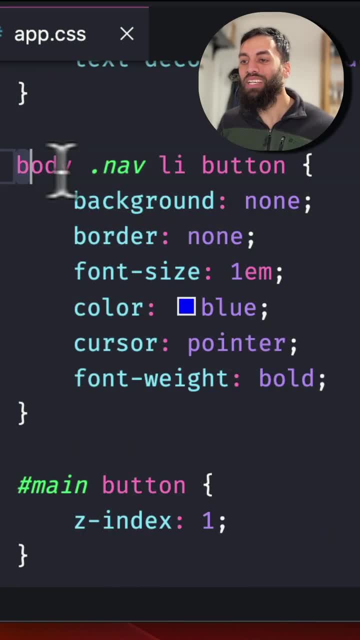 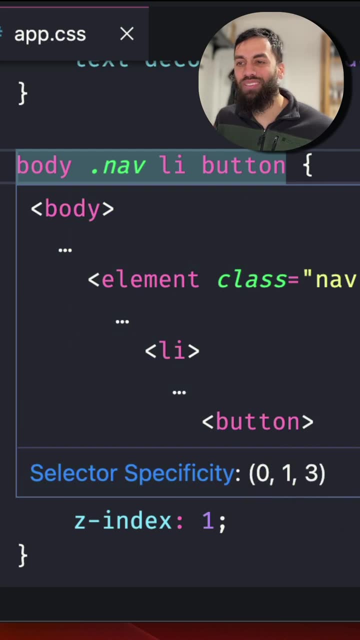 0, 1, 1,. okay, Now look at these two selectors. You might think the first is more specific than the second because there's more parts to it, but the second has hash main, which is an ID portion. So the first selector, 0, 1, 3,. the second selector which has the ID component. 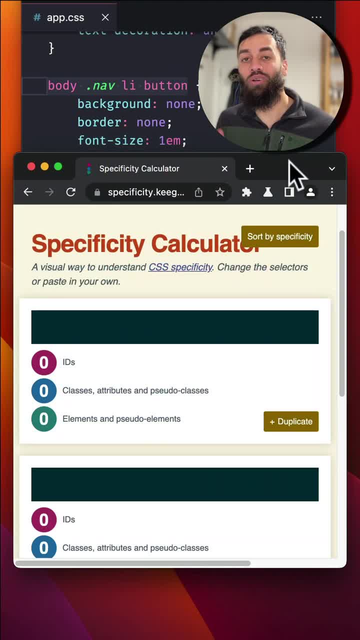 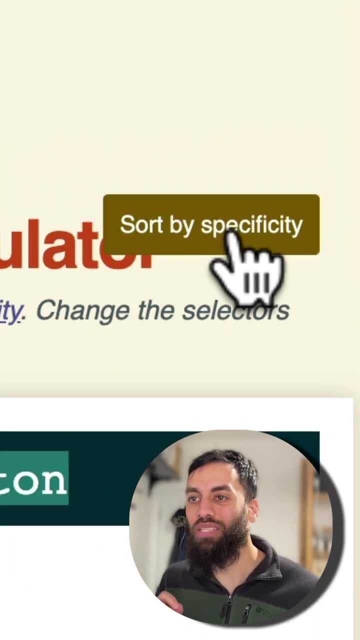 to it 1 0, 1.. Let's paste those selectors into an online specificity calculator. I really like this page as it explains what the different parts of the selector are, Alright, and then sort by specificity. Are our suspicions confirmed? Yes, Hash main carries massive weighting and